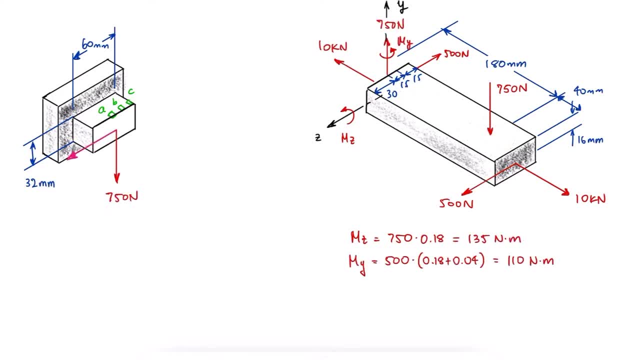 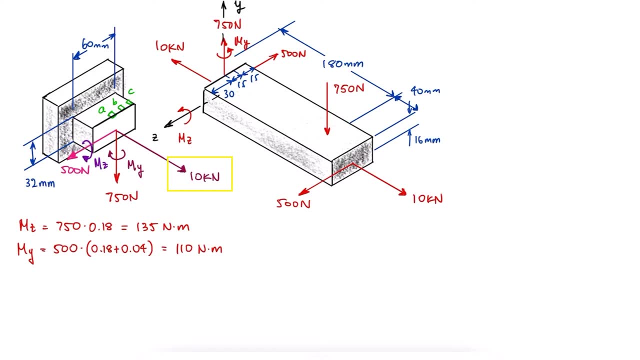 the y-axis We see the reactions with opposite directions as the internal loads on the other side of the cut. Because of the 10 kN load that is perpendicular or normal to the cross-section area, all three elements, A, B and C will be subjected to a positive normal stress due. 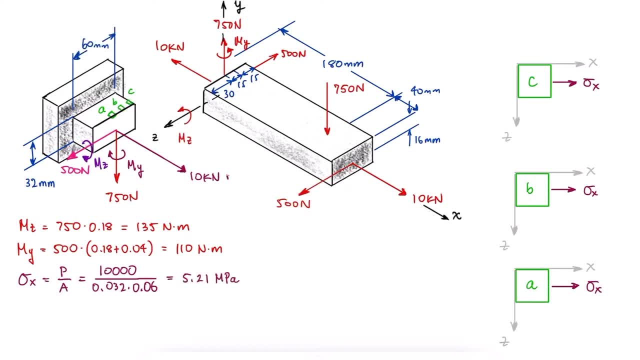 to axial loading in the direction of the x-axis. Since there are no torques, meaning no moment about the x-axis, there are no torsional shearing stresses Due to the moment m sub z, we see that any element on the top surface will be subjected to tension and any element on the bottom surface 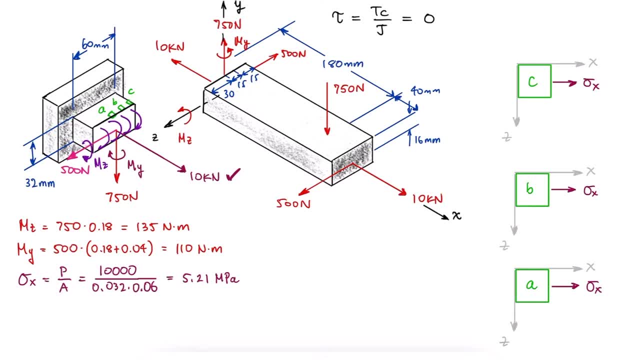 to compression due to the bending. For this reason, elements A, B and C are all subjected to a bending- normal stress- where y is the distance from the neutral axis to the top surface. The second moment of area I is that about the z-axis, which means that the width of 60 mm. 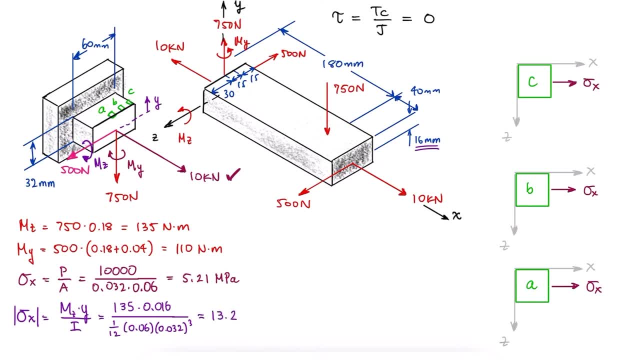 is the base and the 32 mm dimension is the height. Again, this normal stress affects all elements and is found in the direction of the x-axis. The moment about the y-axis will not affect element A, since element A is located on the neutral axis. However, elements B and C will be subjected to a tensile normal stress due. 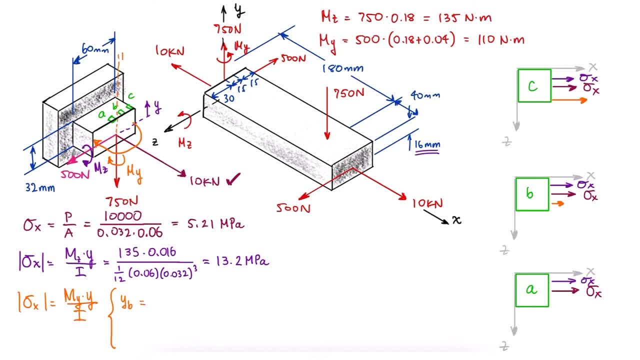 to bending, where yB is the distance from the neutral axis to location B and yC is the distance from the neutral axis to location A, neutral axis to location C. Of course this normal stress at C is higher than at B because C is farther away from the neutral axis. And notice that the second moment of area is that 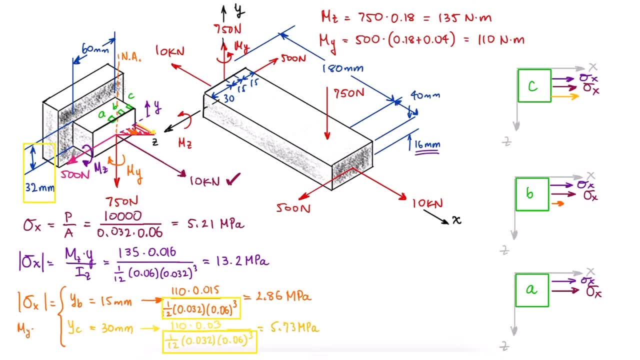 about Y, where the base is 32 mm and the height is 60.. Finally, the 750 N load creates a shearing stress right at the middle of the cross-section area. that becomes zero at the top or the bottom, since at those locations the value of Q would be zero. So the 750 N shear force doesn't have. 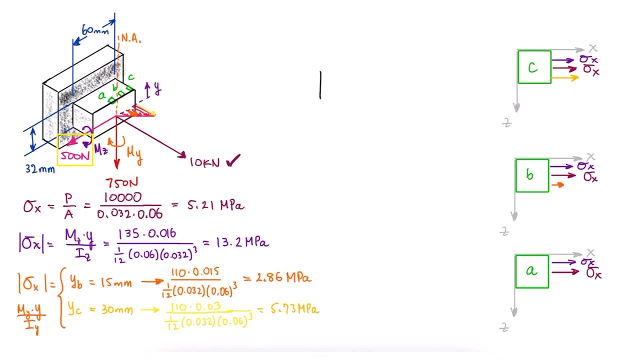 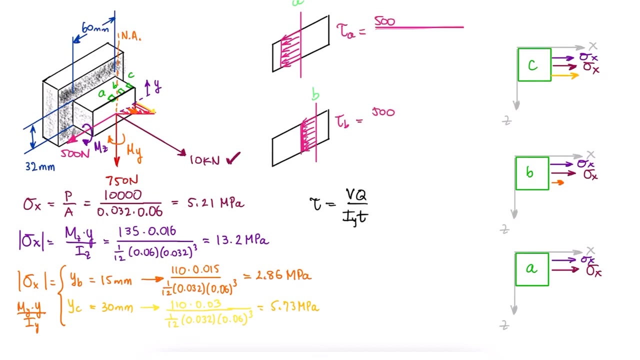 any effect on locations A, B or C, But the 500 N shear load creates a transverse shear stress that is maximum at location A, zero at location C and somewhere in between at location B. V is the 500 N load. I is the second moment of area about the Y axis. T is the thickness. 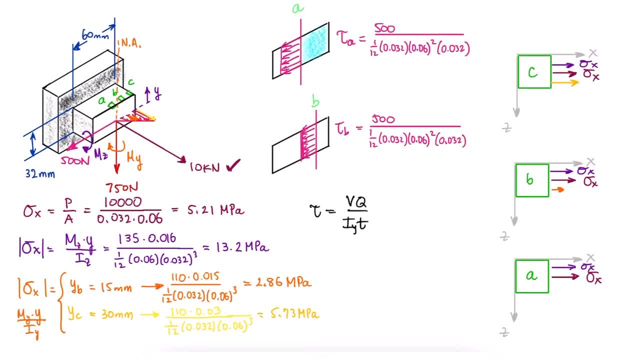 perpendicular to the shear force and V is the second moment of area about the Y axis, In Q, the first moment of area of the region above or below the location of the shearing stress. we are calculating With the Q values being different. for A and B we find the different. 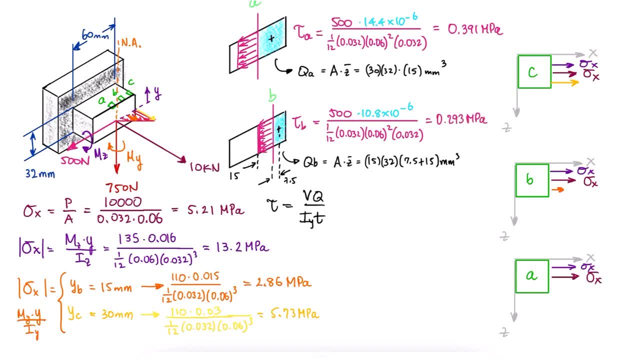 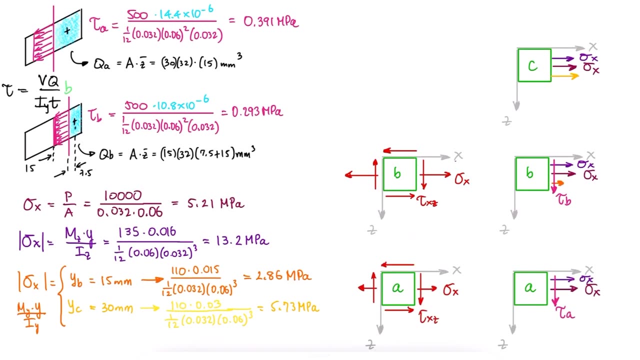 values for the shearing stresses. But in both cases this shearing stress affects the side that is facing the positive X axis and the direction of the vector is the positive Z axis. The resulting normal and shearing stresses are there for a sigma X and a tau X Z for elements. 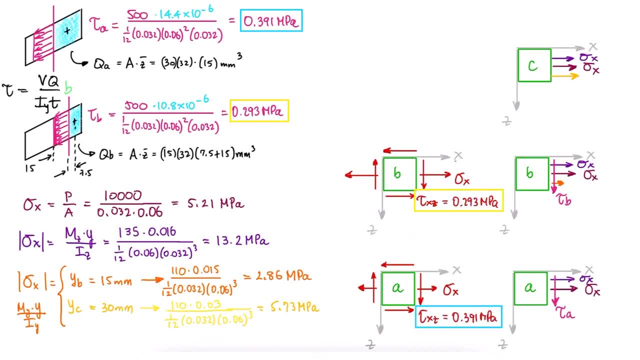 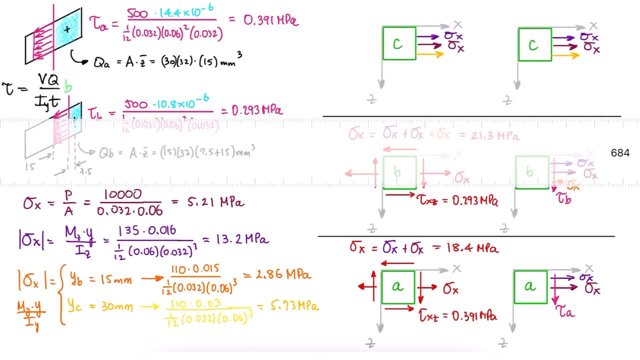 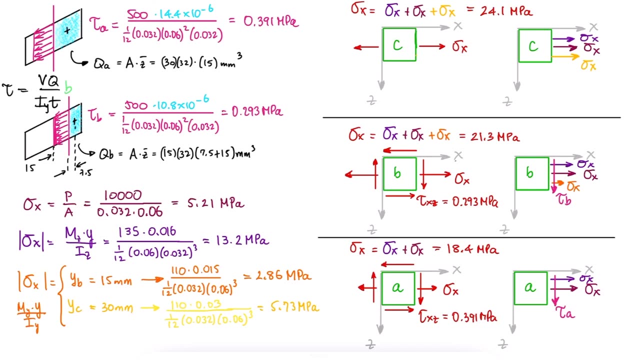 A and B, where the shearing stress is what we just found and the normal stress the sum of the previously calculated normal stresses- 3 for B and 2 for A, and only one normal stress for element C. With these stress states, we would be able to use more circle to find the principal stresses. 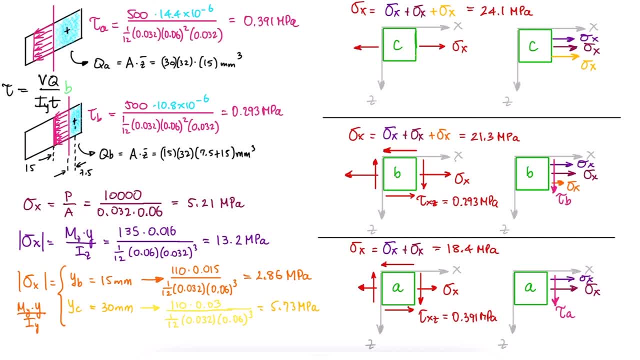 and the maximum shearing stresses for each location: A, B and C. Thanks for watching. 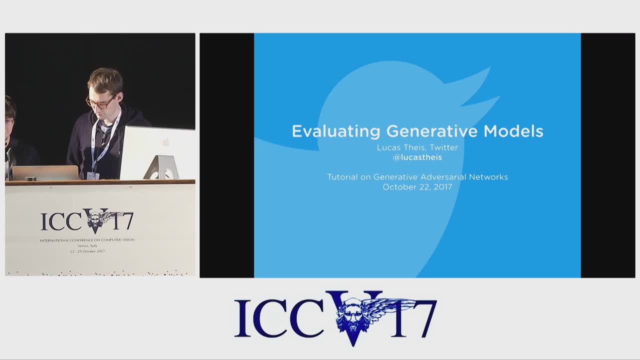 Thanks. Our next speaker is Lucas, who's a researcher at Twitter. He joined Twitter via the acquisition of Magic Pony. He works on a variety of image applications at Twitter And he's here to tell us about a lot of the difficulties associated with evaluating generative models, which a lot of areas of machine learning. we understand what metrics you want to improve and the difficulties, and how do we improve those metrics For generative models. it's actually conceptually very difficult. 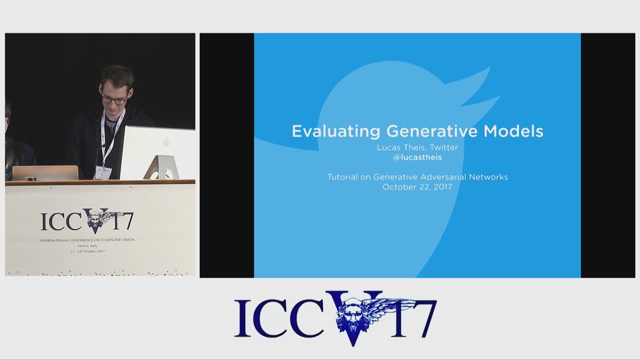 To figure out what we actually want, to even measure, And he's here to guide us through a lot of those difficult issues. Hello everyone. Yes, Ian said this talk is going to be about the evaluation of generative models And, just to be clear, it's not going to be so much about which objective functions you should choose during training, although, of course, evaluation and training are closely related.